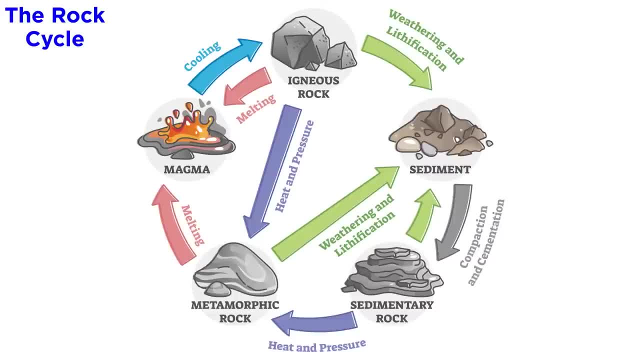 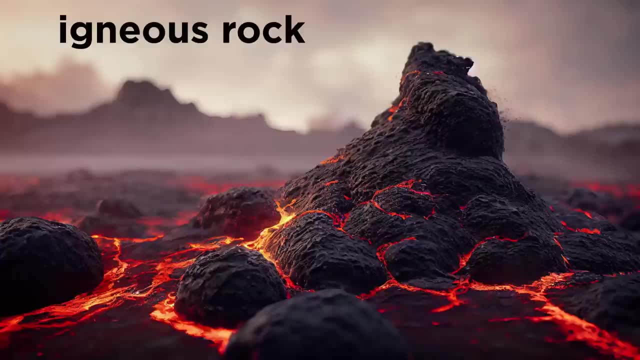 This involves the formation and destruction of rock throughout geologic history. For example, in Earth's early history, all rocks at the surface were igneous. having formed from the cooling of liquid magma and pushed up to the surface Over long periods of time, rain and 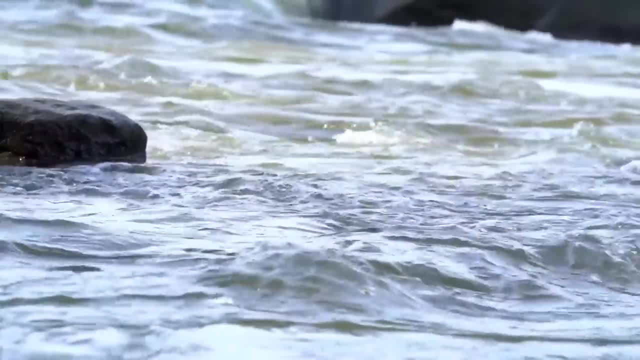 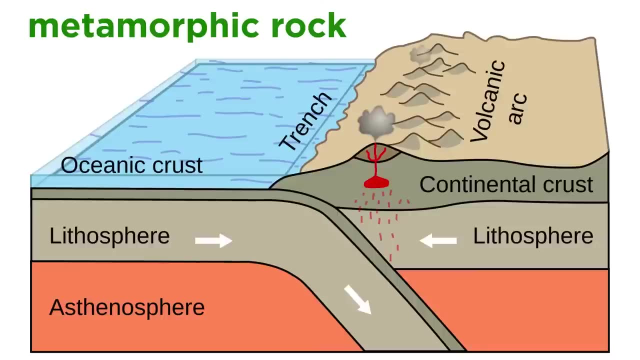 wind would break these rocks apart and transport their sediments to the oceans, where they would be buried and later lithified into sedimentary rocks In parts of the world where two plates were moving together. these original igneous rocks were metamorphosed by the heat and pressure of 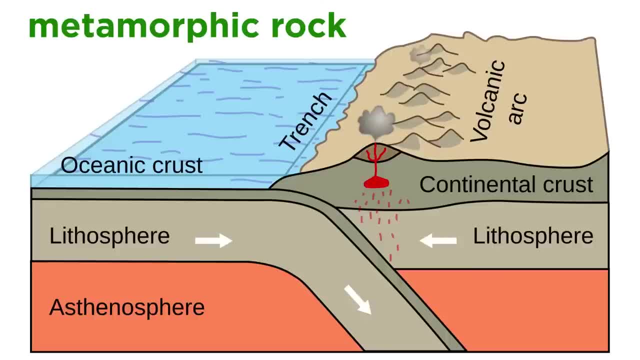 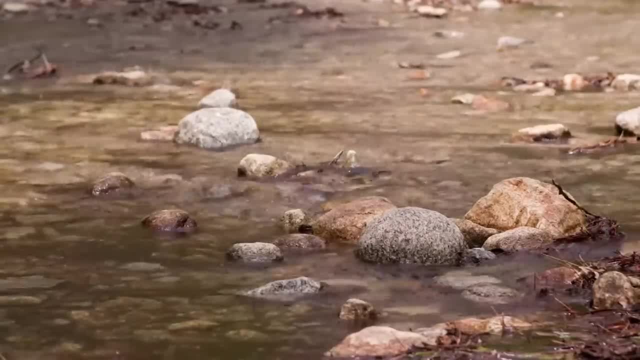 collision and uplifted to form mountains containing metamorphic rock. And, just as before, these rocks were broken down and their sediments transported to sedimentary basins. These new sedimentary rocks were then transformed into sedimentary rocks, which were then moved to. 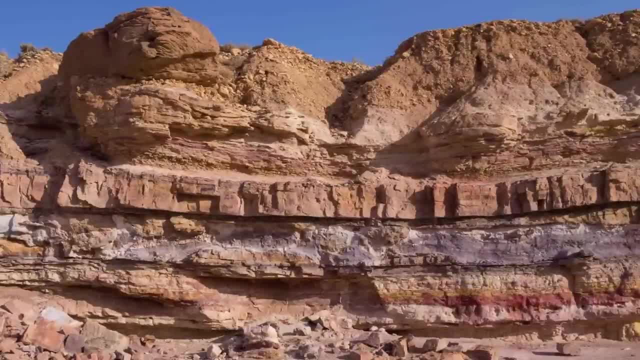 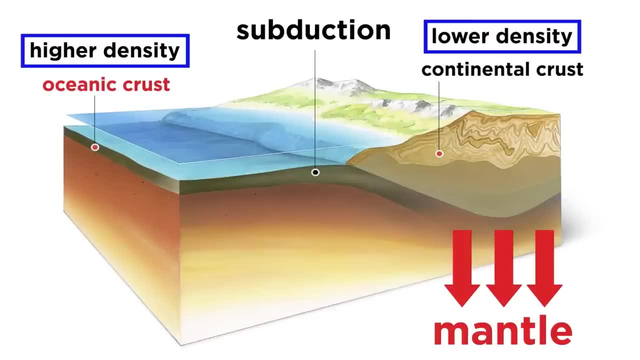 rocks that would later be uplifted and exhumed, where they would again be attacked by the wind and rain, broken into sediment and transported to a brand new sedimentary basin In parts of the world that were experiencing subduction. the original rock in the subducting slab was returned to the 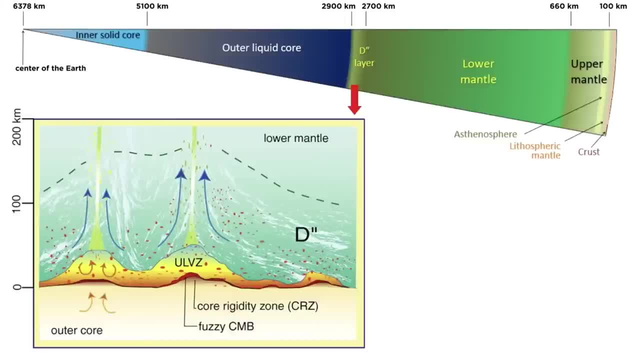 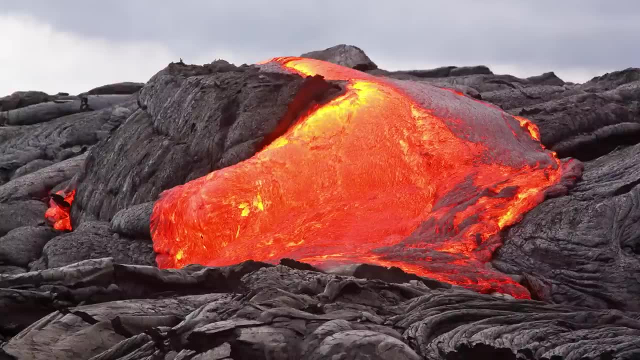 mantle, where it would presumably sink to D double prime and later rise to form a mantle plume, which would melt, create a volcano and erupt lava to form a brand new igneous rock that perhaps shares a few silicon or oxygen atoms, in common with the rock from the previous iteration of the. 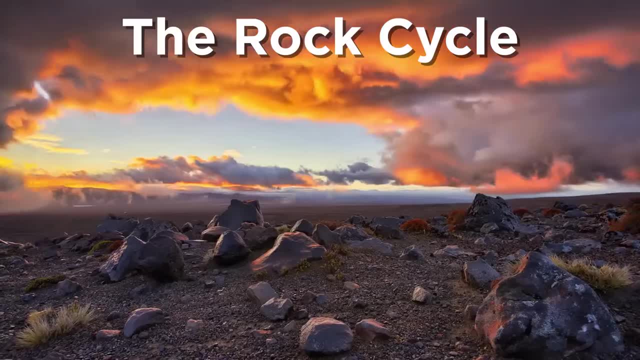 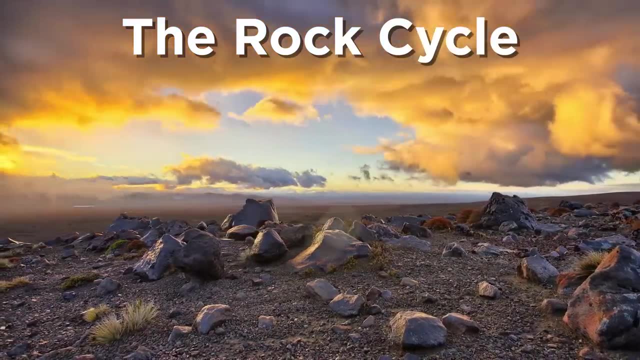 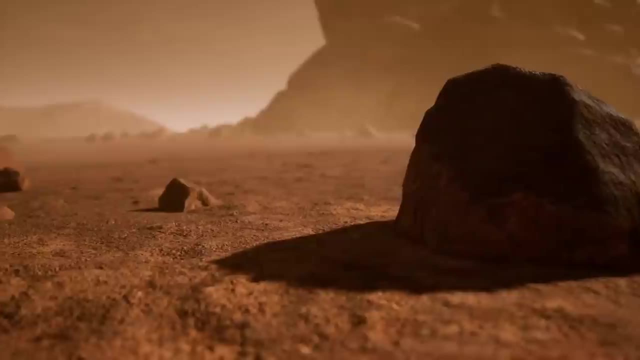 cycle, And then the whole show begins again. It is by these processes, which are collectively referred to as the rock cycle, that earth continuously recycles. geologic material and, in some cases, mineral grains from the primordial earth have survived over four billion years of the rock cycle and exist today as parts of ancient sedimentary rocks. 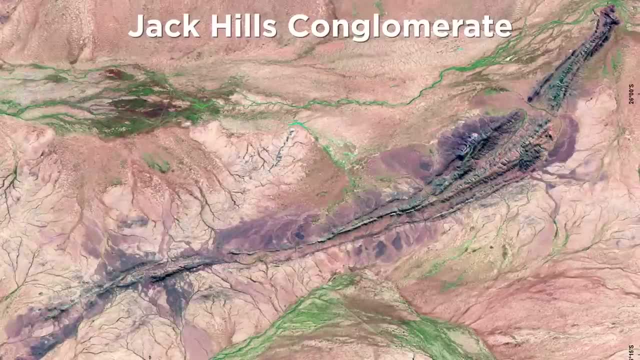 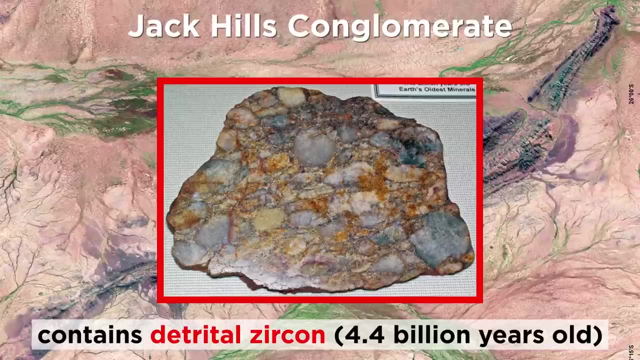 A famous formation of the rock cycle is the rock cycle of the earth, which is the rock cycle of the sun. This formation in Australia, called the Jack Hills Conglomerate, contains detrital zircon, which is a particularly durable mineral that is over 4.4 billion years old. 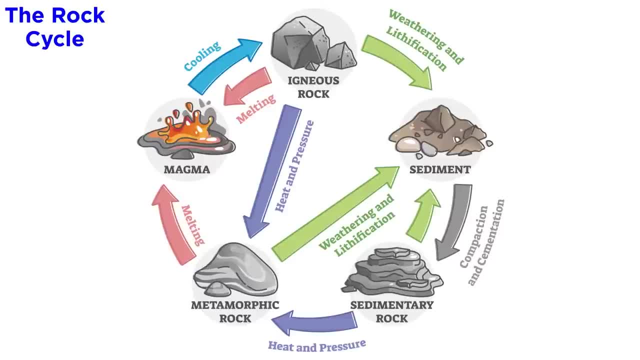 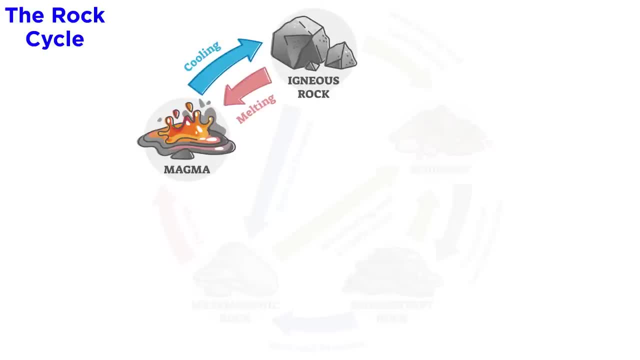 We can look at an image like this to summarize all of the possibilities within the rock cycle at once. We start with magma which cools to form igneous rock. This could melt to form magma again, or it could experience weathering and erosion to form sediments which can compact and 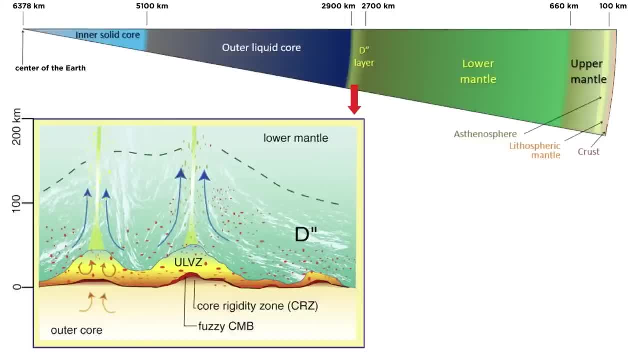 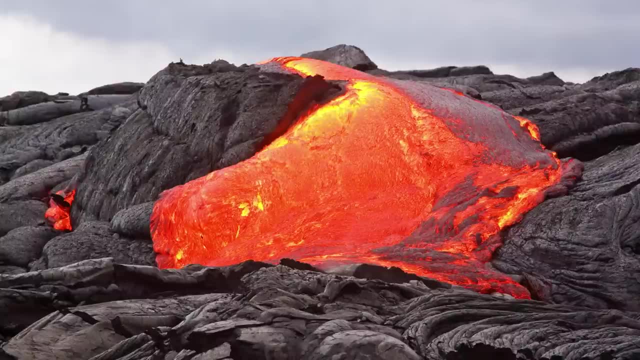 to the mantle, where it would presumably sink to D double prime and later rise to form a mantle plume, which would melt, create a volcano and erupt lava to form a brand new igneous rock that perhaps shares a few silicon or oxygen atoms, in common with the rock from the previous iteration of the. 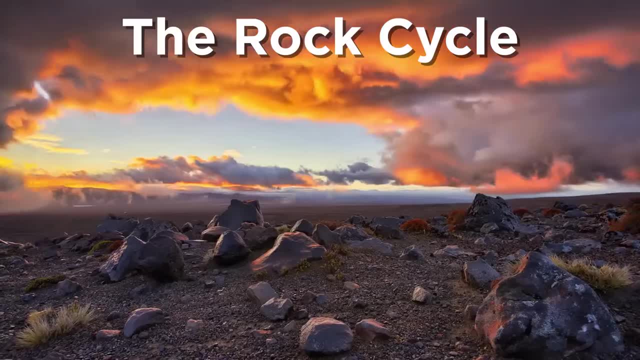 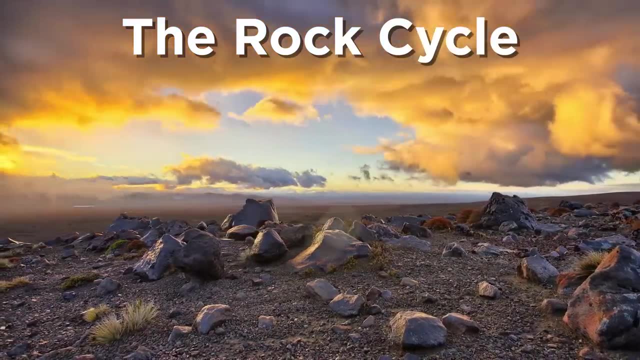 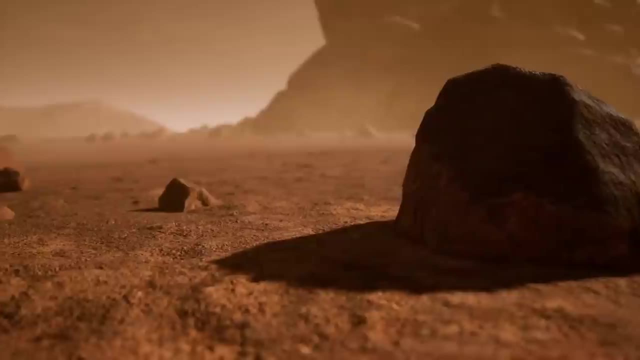 cycle, And then the whole show begins again. It is by these processes, which are collectively referred to as the rock cycle, that earth continuously recycles. geologic material and, in some cases, mineral grains from the primordial earth have survived over four billion years of the rock cycle and exist today as parts of ancient sedimentary rocks. 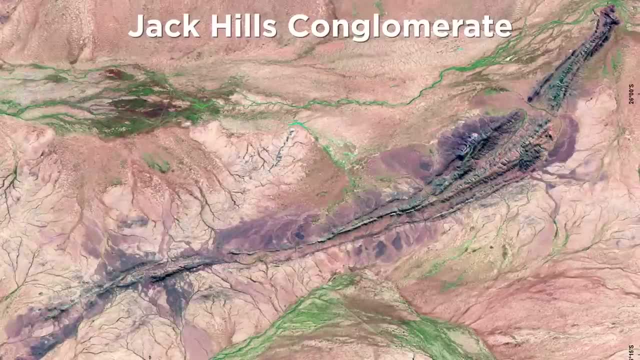 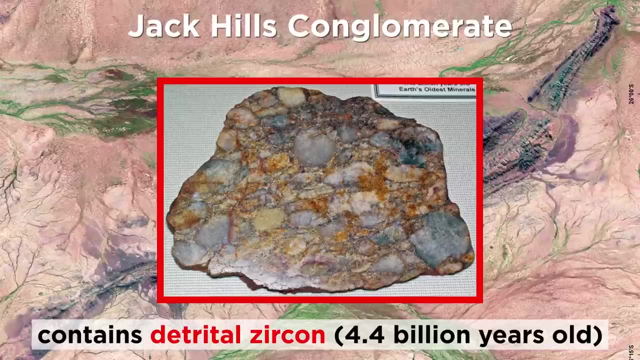 A famous formation of the rock cycle is the rock cycle of the earth, which is the rock cycle of the sun. This formation in Australia, called the Jack Hills conglomerate, contains detrital zircon, which is a particularly durable mineral that is over 4.4 billion years old. 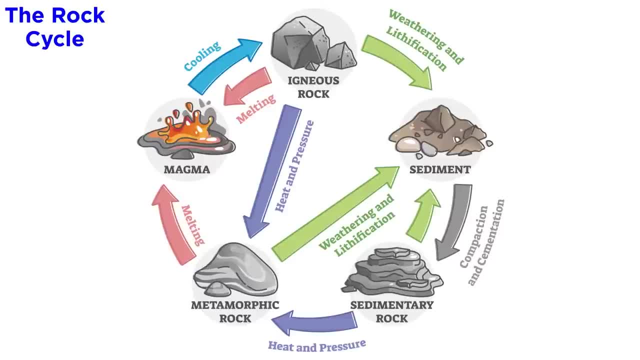 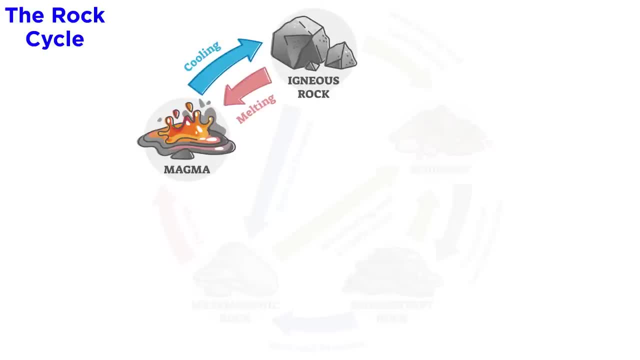 We can look at an image like this to summarize all of the possibilities within the rock cycle at once. We start with magma which cools to form igneous rock. This could melt to form magma again, or it could experience weathering and erosion to form sediments which can compact and 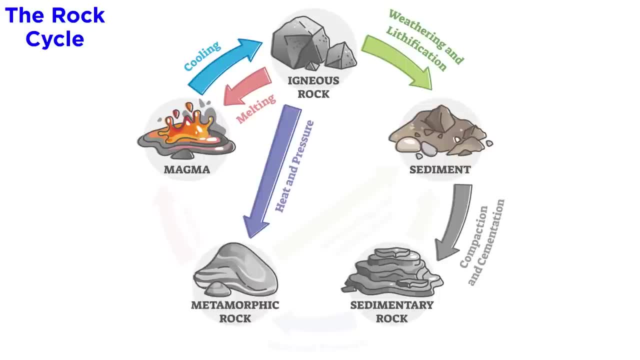 melt to form sedimentary rock. Igneous rock can also experience high heat and pressure to form metamorphic rock. Sedimentary rocks can do the same thing. if they are also subjected to such high heats and pressures, Then both sedimentary rock and metamorphic rock can experience weathering. 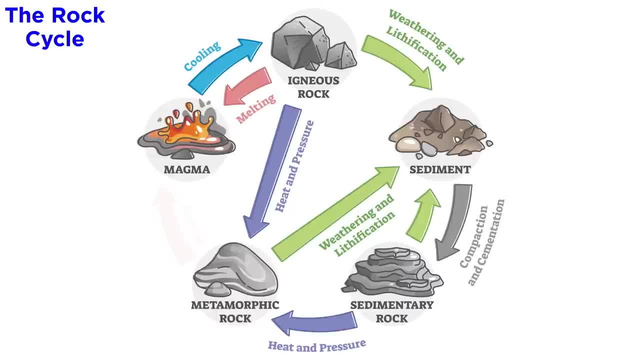 and erosion to produce sediments just like igneous rock, and this sediment will eventually compact to form still more sedimentary rock. And metamorphic rock can also melt, just like igneous rock, to produce magma and return to the source of it all. 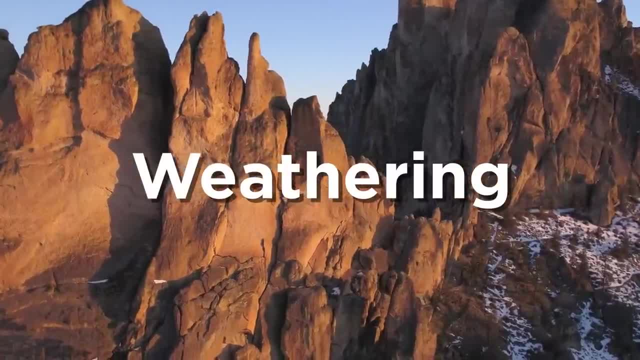 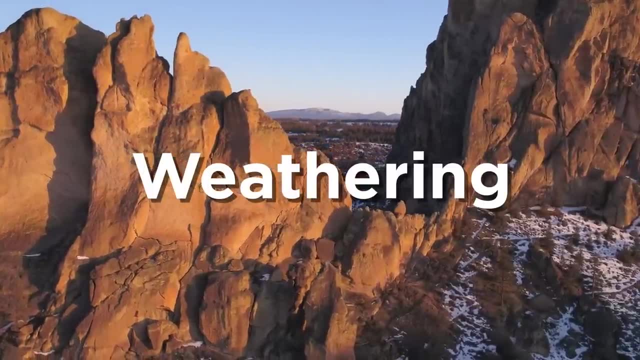 In describing the rock cycle and in talking about the production of sediments in general. we mentioned weathering many times, but we haven't gone into much detail regarding these processes. So let's move forward and talk about precisely how weathering and erosion transform rocks into sediment. 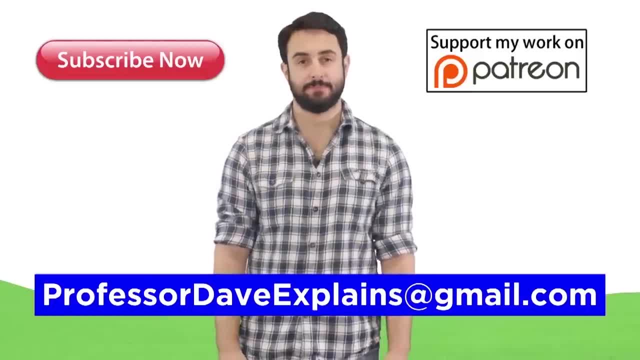 As always, feel free to email me at professordaveexplains at gmailcom. 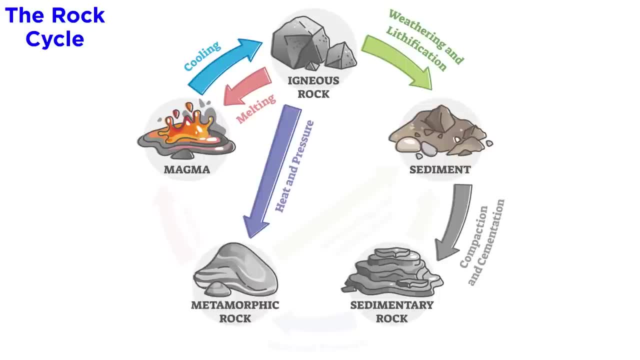 melt to form sedimentary rock. Igneous rock can also experience high heat and pressure to form metamorphic rock. Sedimentary rocks can do the same thing. if they are also subjected to such high heats and pressures, Then both sedimentary rock and metamorphic rock can experience weathering. 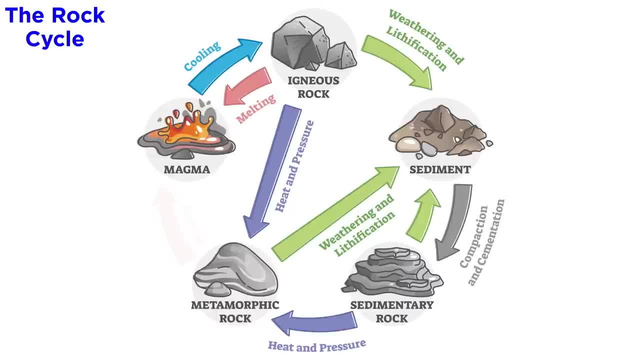 and erosion to produce sediments just like igneous rock, and this sediment will eventually compact to form still more sedimentary rock. And metamorphic rock can also melt, just like igneous rock, to produce magma and return to the source of it all. 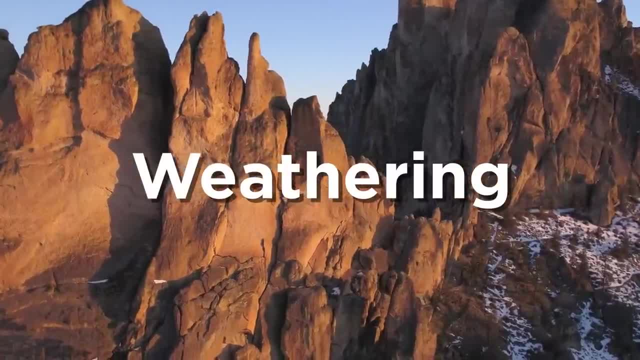 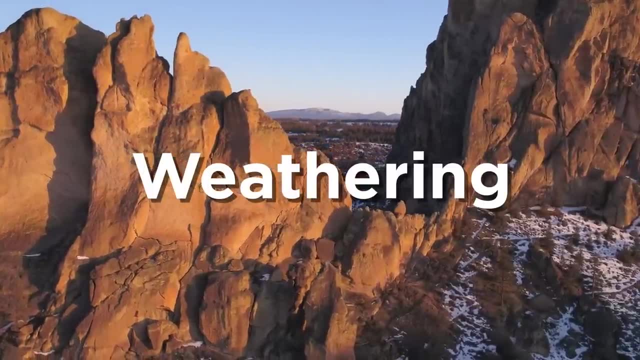 In describing the rock cycle and in talking about the production of sediments in general. we mentioned weathering many times, but we haven't gone into much detail regarding these processes. So let's move forward and talk about precisely how weathering and erosion transform rocks into sediment. Feel free to email me professordaveexplains at gmailcom. 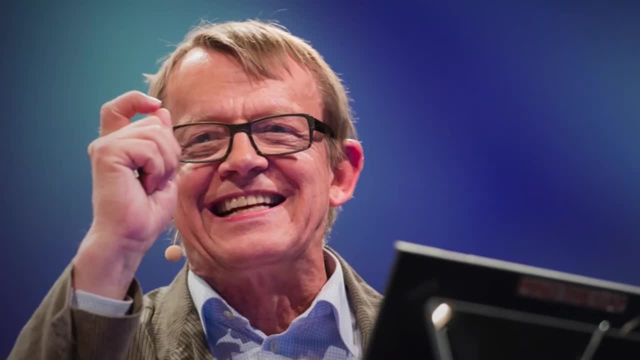 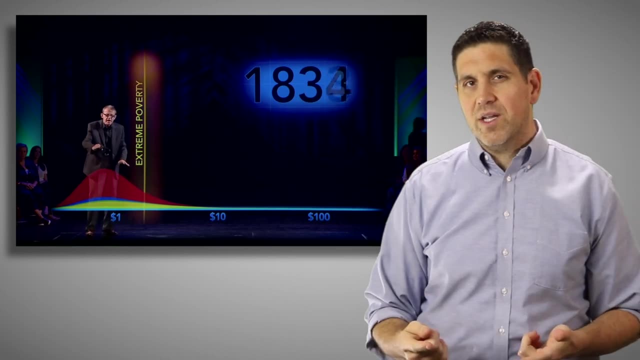 Hey Internet. this is Jacob Clifford, and welcome to my YouTube channel. The late great Hans Rosling, a statistician and global health professor, liked to ask his audience questions before his TED talks, And he found some interesting results. So with that in mind, I have two questions for you. Good luck. 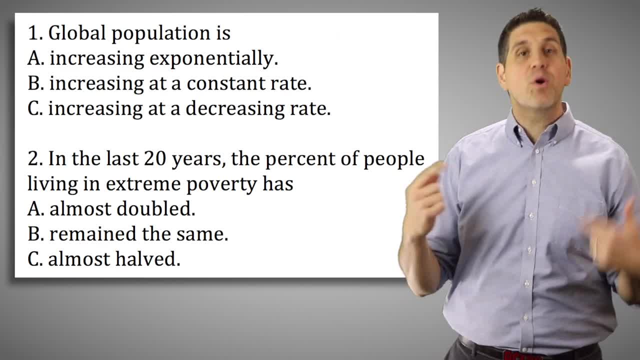 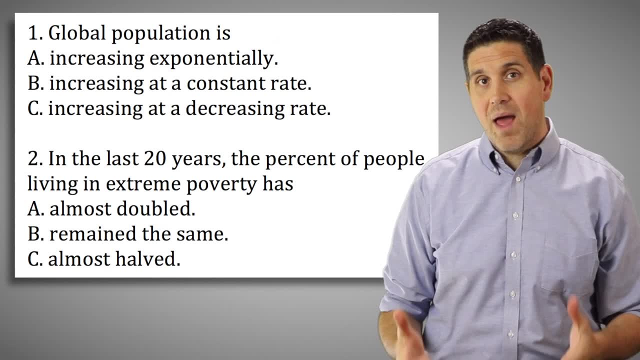 What Rosling found was that most people get these questions wrong because they have preconceived ideas about the world. They think the world is the same as it was 50 or 20 years ago. If you ask around, you'd be surprised to find out how many people don't know the population. 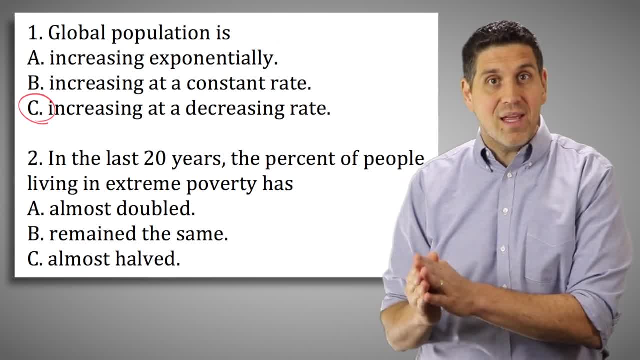 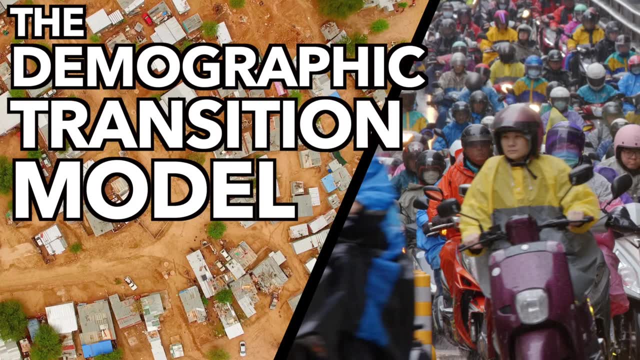 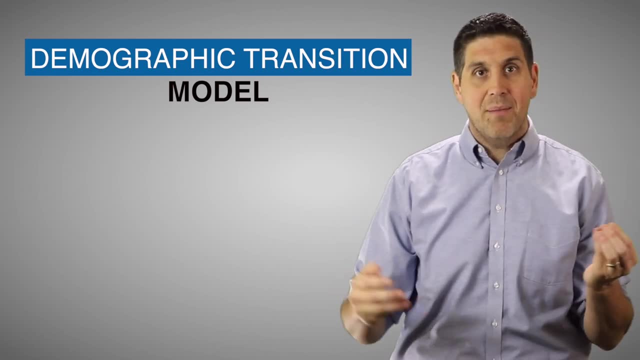 is increasing at a decreasing rate or the extreme poverty is significantly decreasing And there's even fewer people that can explain why that's happening. In this video, I'm going to connect economic development to something called the demographic transition model. It's going to show three different things that change over time. The 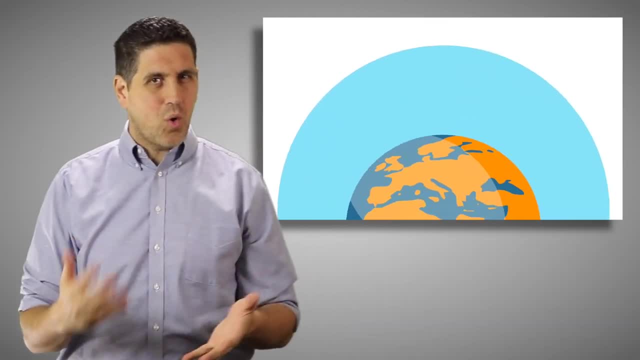 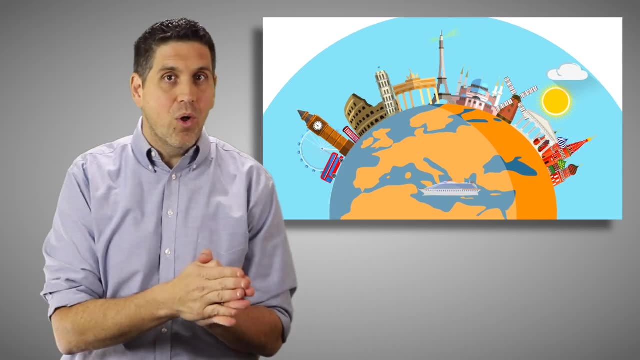 birth rate, the death rate and the total population. To give it some historical context, I'm going to focus on the US and Western Europe, But remember every country goes through this process, although some might not fit the mold, and some transition quicker than others. 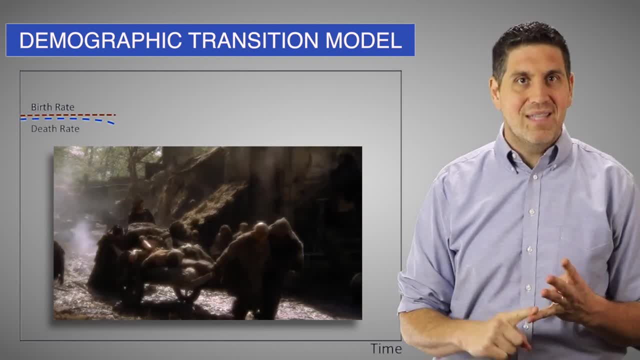 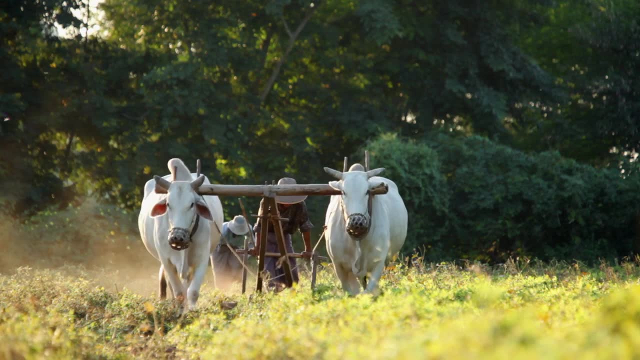 hospitals or medicine And life was just basically hunger, disease, war and death, A lot of death. And there really wasn't much change in the world. There really wasn't an economy, because most of it was subsistence farming where people were growing.